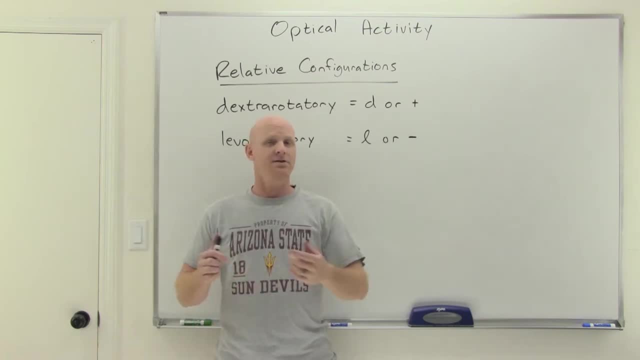 you'll be on the hook for everything we do in this chapter, including a lovely calculation, So one of the few calculations you might see in an organic chemistry course. Now, if this is your first time joining me, my name is Chad, and welcome to Chad's Prep, where my goal is to make science. 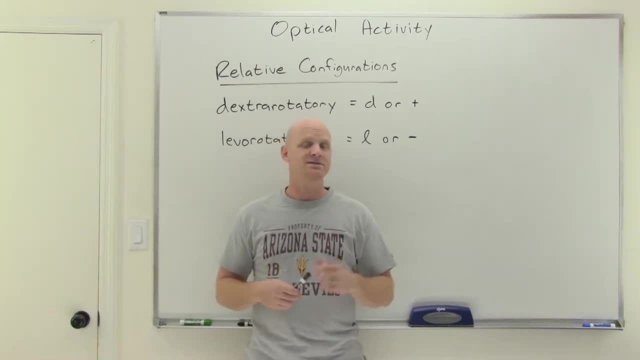 both understandable and maybe even enjoyable. Now this is my brand new organic chemistry playlist. I'll be releasing these lessons weekly throughout the 2020-21 school year, So if you don't want to miss one, subscribe to the channel. click the bell notifications. 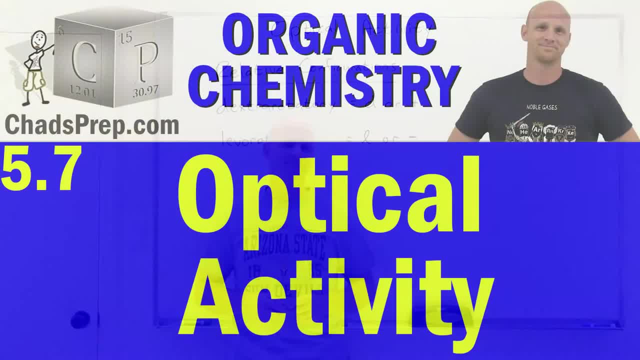 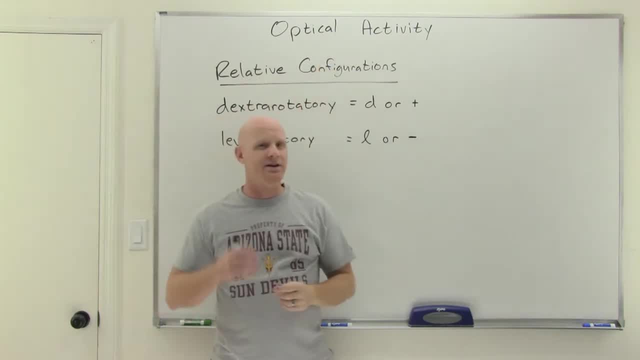 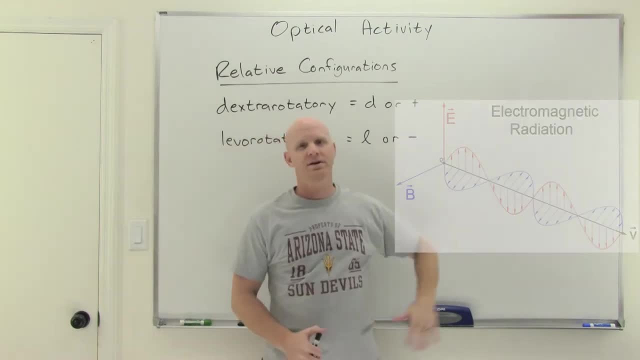 you'll be notified every time I post another lesson. All right, so we introduced optical activity a little bit earlier in this chapter and we talked about what's called plane polarized light, And I'll put up a little diagram on the board here. 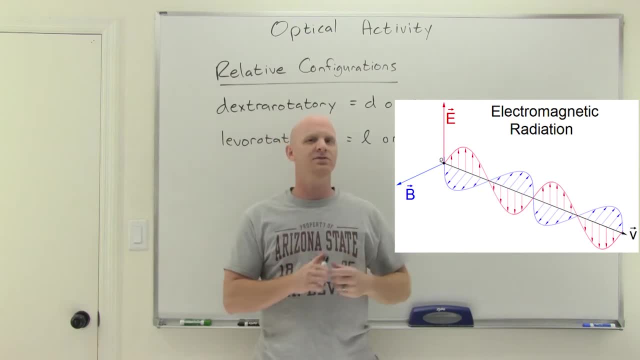 So, but light has both an electric field and a magnetic field associated with it, and they're orthogonal to each other. They're oriented 90 degrees apart from each other. And so, as a result, though depending on their vectors- in this case- and you'll see them in a physics class, but depending 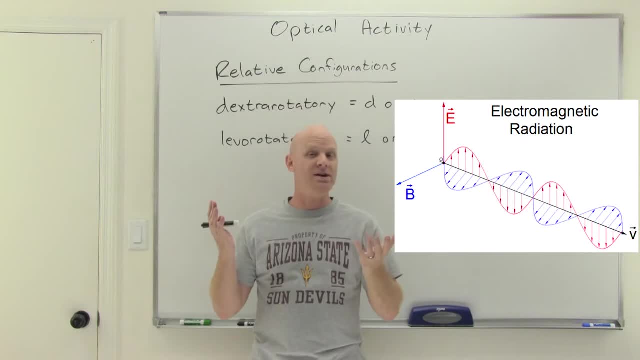 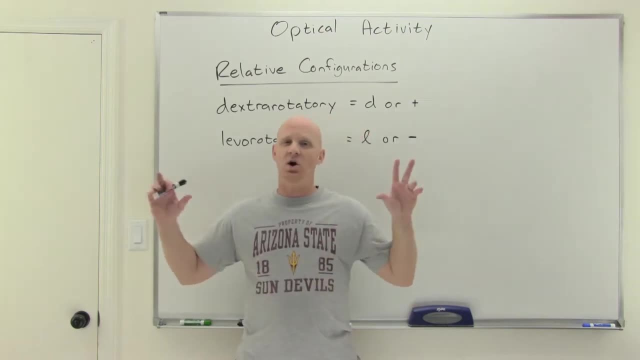 on which way they're oriented. so it turns out light has a specific orientation associated with it. So every photon of light has an orientation associated with it, And when you've got unpolarized light, it just means that all your photons have any kind of orientation, just random assortment. 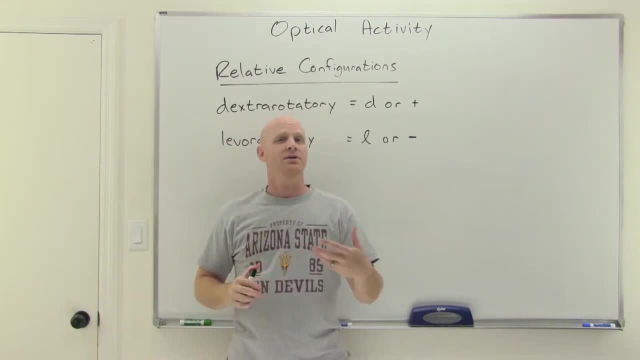 of all the different orientations around 360 degrees. But you can run that through what's called a polarizing filter- and polarizing sunglasses are polarizing filters- And what happens is it's going to block out a lot of those different orientations so that you largely have 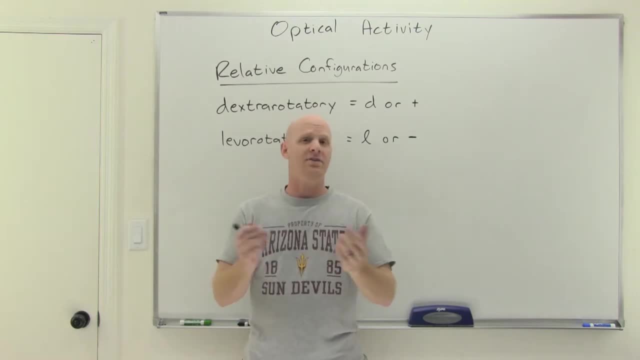 just a single orientation And we call that then at that point plain polarized light. And funny thing that happens is when you shine plain polarized light through a solution that contains a compound that is chiral, it gets rotated one way or the other And the different enantiomers 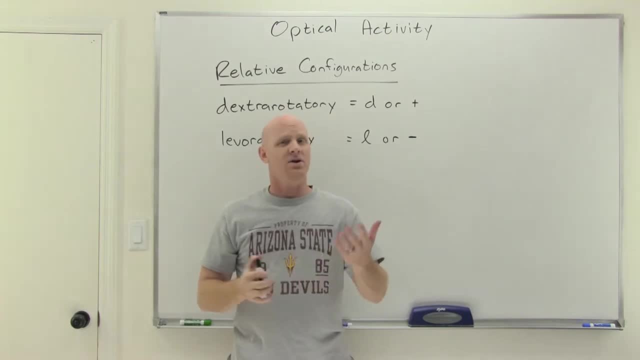 of a compound rotate it In opposite directions. So, in contrast that with achiral compounds, achiral compounds don't rotate it at all. If it goes through with a vertical orientation, it comes out the other side with still a vertical orientation, And so, as a result, we refer to chiral compounds as being 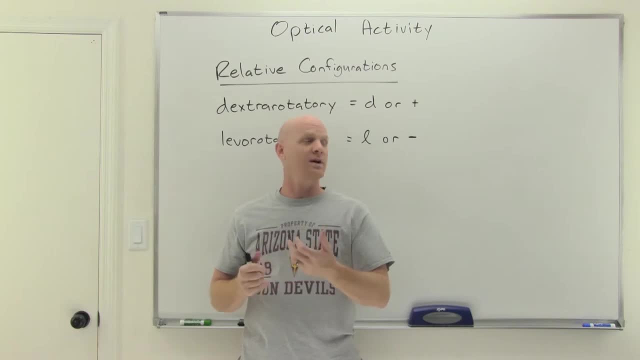 optically active, They rotate plain polarized light. And then we refer to achiral compounds as optically inactive. They don't rotate plain polarized light. And we also learned a new vocabulary. that was racemic mixture, And that's when you've got a 50-50 mixture of enantiomers. 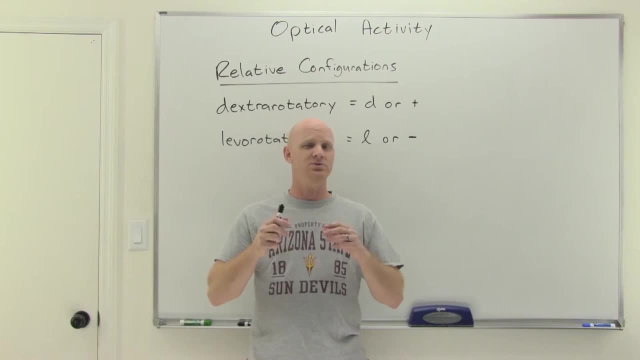 that solution would also be optically inactive. Half the molecules in that solution want to rotate light one way. half the molecules want to rotate light the other way, And so, on average, light doesn't get rotated by a racemic mixture either. So either you know, individual enantiomer is. 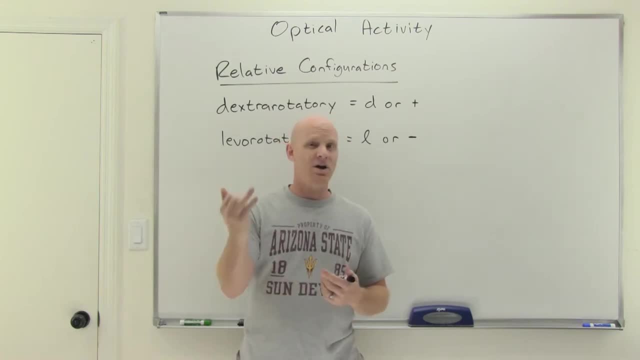 optically active, So, whereas an achiral compound or racemic mixture optically inactive. We'll also find out that if it's not exactly 50-50, even if it's like a 51%- 49%, that that solution would. 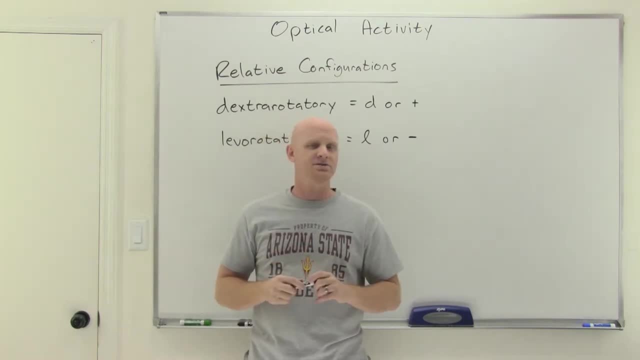 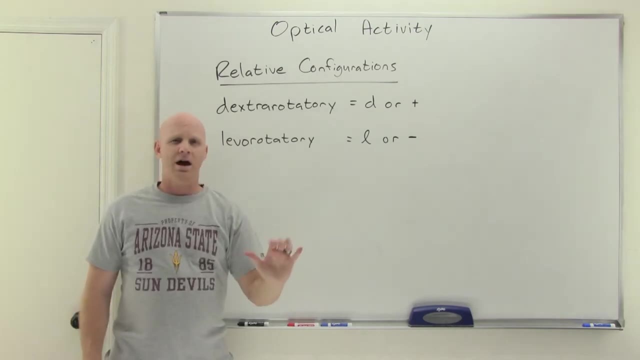 be a little bit optically active as well, And we'll kind of cover some calculations associated with that here in a little bit also. So first I'm going to talk about what are called relative configurations. Now earlier in this chapter we already talked about absolute configurations. 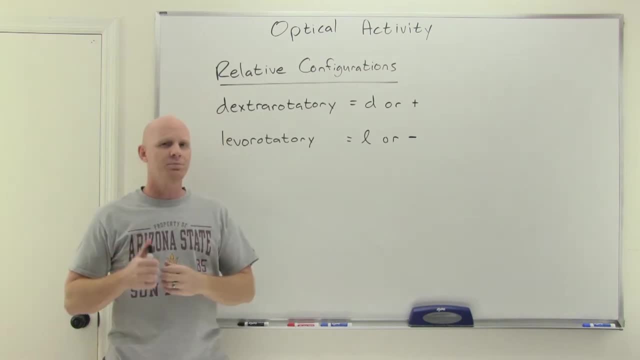 assigning R and S And we learned the Kahn-Ingold pre-log system for assigning priorities and learned that when your number four priority is in the back, a right-handed turn is R and a left-handed turn is S. Okay, great, You can totally tell. you know if a structure is R or S based on looking. 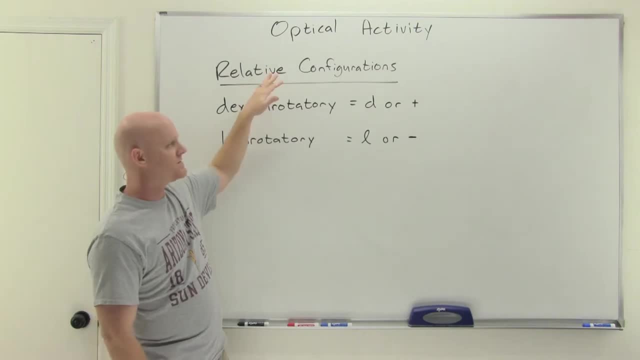 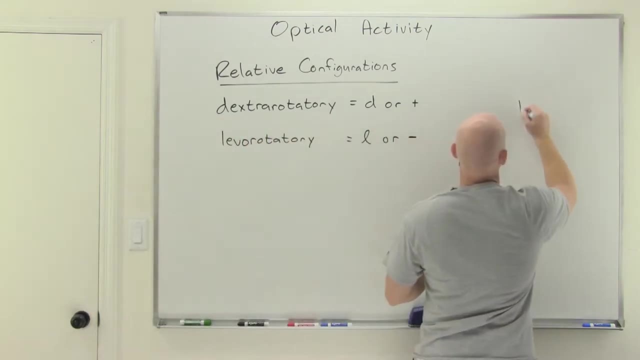 at the structure. So not true for what we're going to call relative configurations, And these are done with which way they rotate: plane polarized light. So let's say we've got light here and we're going to put it on the vertical here at zero degrees And that light's going to get. 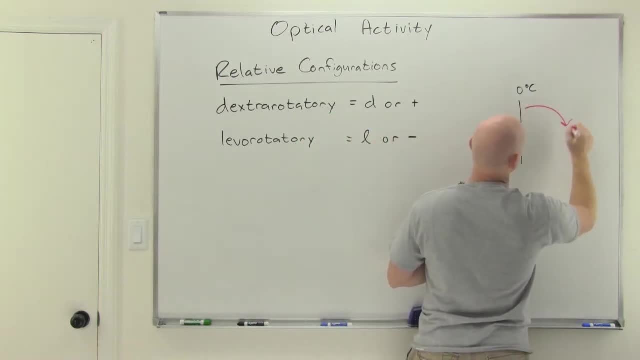 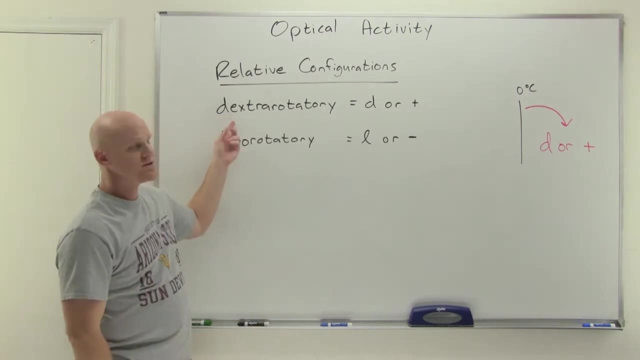 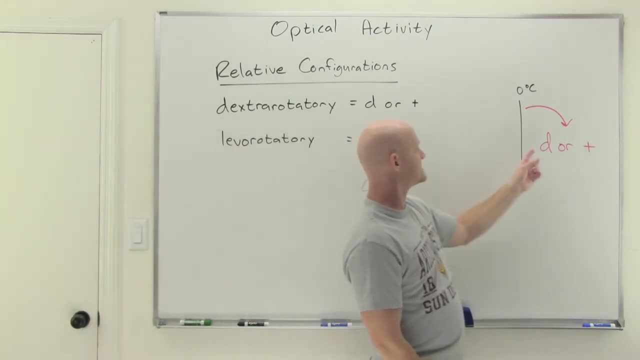 rotated in one of two directions. If it gets rotated off to the right, then we either call it D or plus, both designations for this relative configuration, And the D here stands for dextrorotatory, which just simply means right rotating. And again, D and plus are really synonymous in this case. 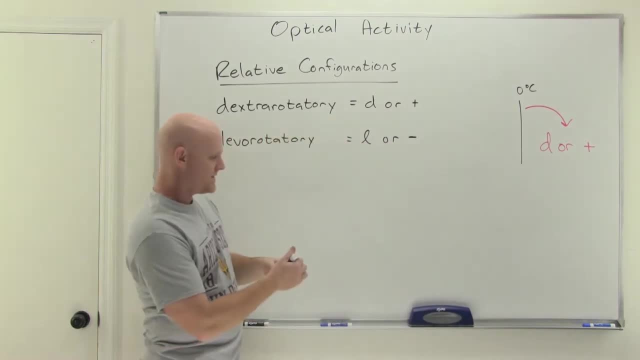 and both represent this relative configuration. So we're going to talk about that in a little bit. Now, on the other hand, if the light gets rotated to the left, then we're either going to call it L or minus. Cool, Now here's the deal. One enantiomer is always going to be the D or plus isomer, And 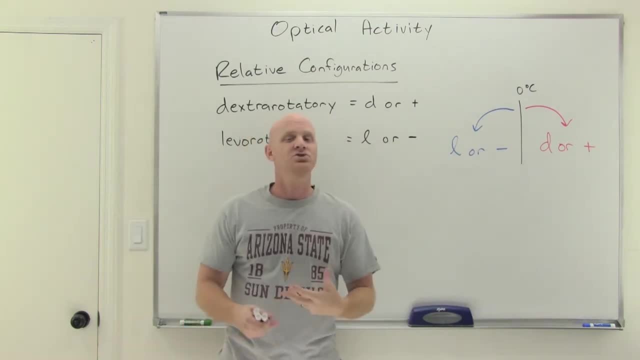 the other enantiomer is going to be the L or minus enantiomer. Now here's the problem is, you can't tell which one is which by looking at the structure. So notice, you can figure out R and S, the absolute configurations, by looking at the structure You can't figure out these relative. 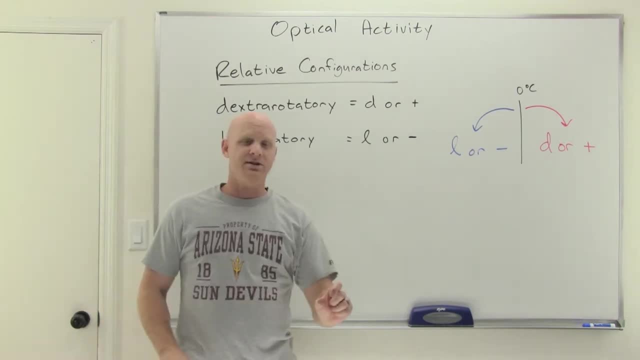 combinations by examining a molecule structure. What you can do is stick that lovely compound in a solution and put it in a polarimeter And then the polarimeter will figure out measure which way the light gets rotated. So you have to use a machine to figure it out. There's no way to just look at. 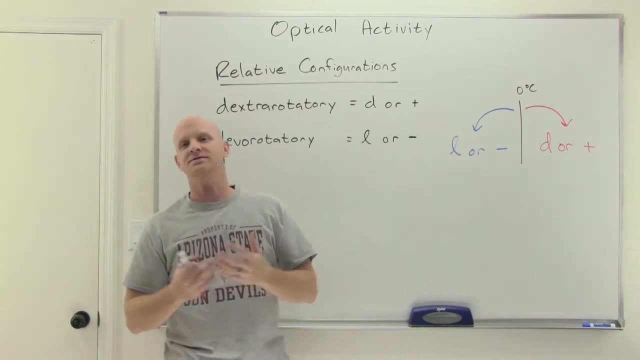 the structural molecule and just like. well, let me think here, Let me do some calculations. It's not going to work that way. So one thing to note then, because you can look at a structure and assign R and S, but you can't look at a structure and assign D or L. there's no connection between. 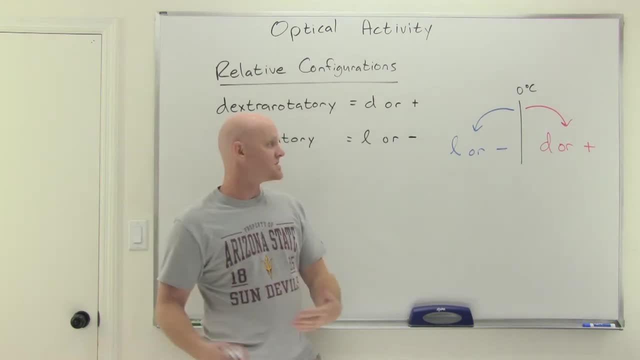 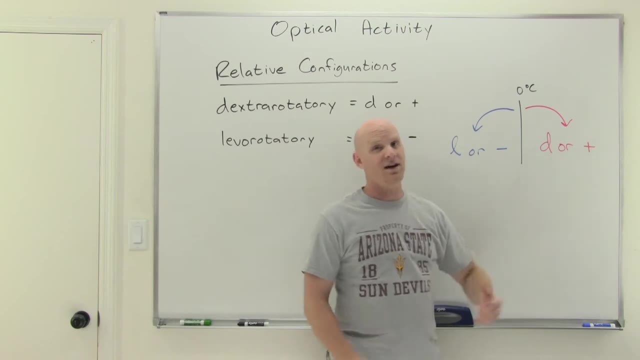 the two. So for some enantiomers the R isomer ends up being the L or minus isomer. For other compounds the R isomer ends up being the D or plus isomer. There's no connection there. What you do know. 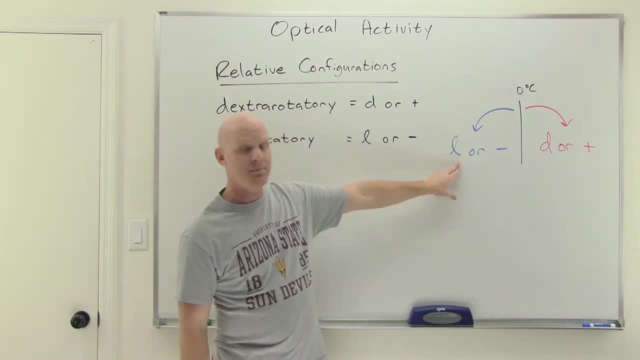 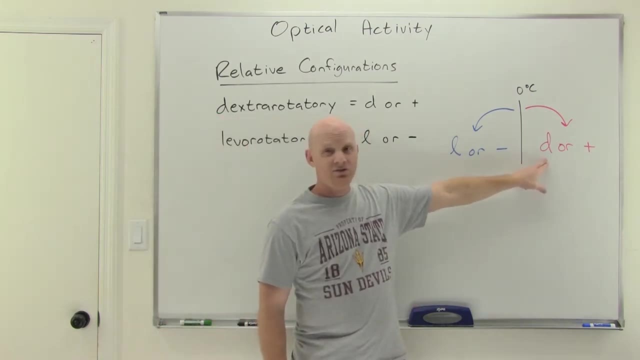 though, is that you're always going to have two enantiomers, And so if I told you that R happened to be the L, the level rotatory isomer, well you'd know, for that specific compound, then the S would correspond to the D or plus isomer. So you always know they're opposites. but until I tell you, 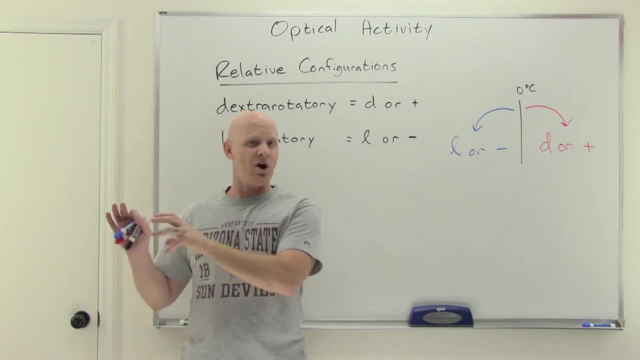 one, you don't have a clue. But if I do give you one of them and show you the connection between R and S, the absolute configuration, and these D and L, these relative configurations, once I give you one, you know, the enantiomer is just the opposite. So keep in mind, there's also 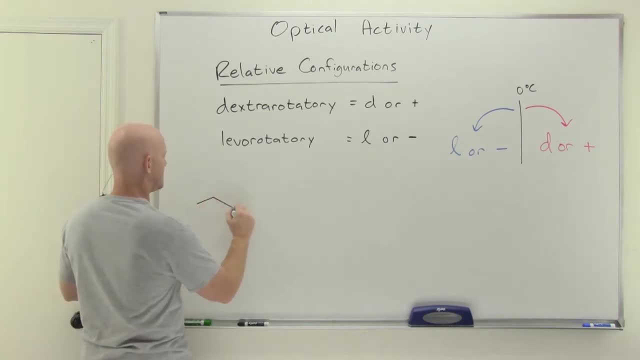 no connection if the molecules look fairly similar. So if I give you this guy here and I tell you that in this case that he is the level rotatory isomer, well then you'd know that his mirror image would end up being the. 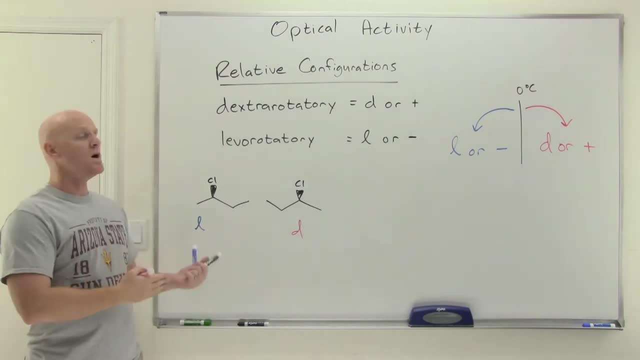 dextrorotatory isomer. So only because I gave you one, could you figure out the other? Now, if I gave you both of this, you know this kind of thing and I said, well, what if you change? 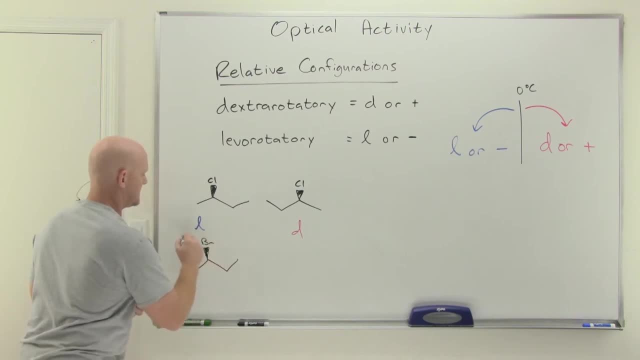 out that chlorine for a bromine And then I say: what isomer is he, What relative configuration is he? And your appropriate answer should be: I have no freaking clue. So again, even though these structures are really close, they're totally different: chiral centers And this. 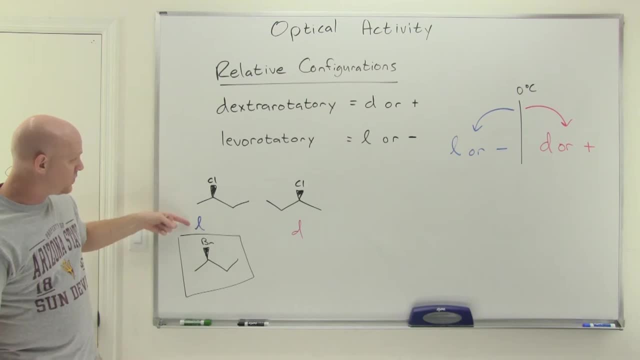 one. you just have no idea which way he's going to rotate light. Again, if I give you one and connect, you know this guy and this guy, you're going to have no idea which way he's going to rotate light. And if you connect this guy with L, then you know his enantiomer is D. But if I just 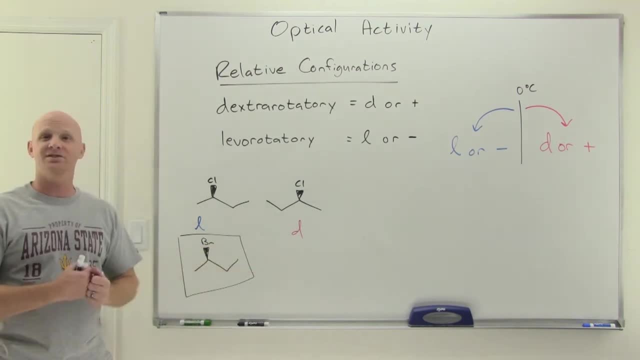 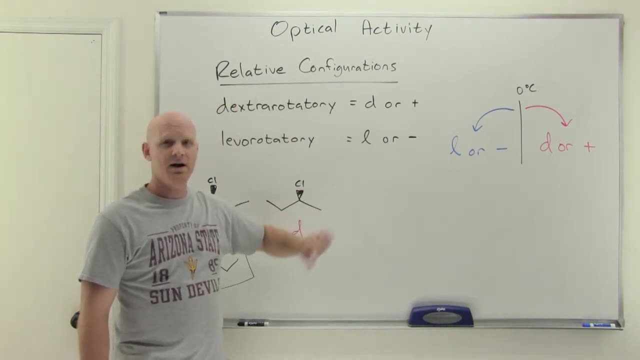 give you one chiral compound and say which way does it rotate light? You should just say I don't know. All right, so those are our relative configurations here, And back in the day they used to name your different enantiomers using these. So it turns out back in the day 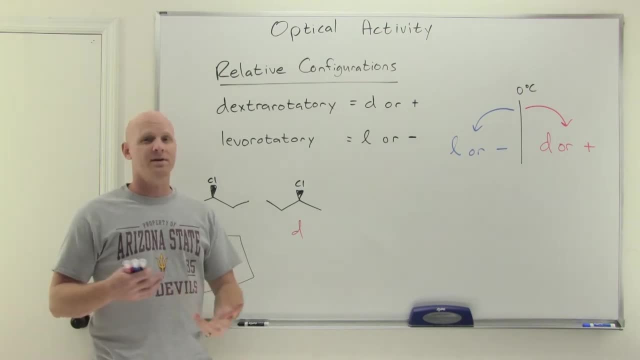 before we really got using NMR extensively and stuff like that, they had a really difficult time figuring out which structure the R or the S actually matched up with which rotation. So it was a big problem. But now that we've got, you know, NMR and stuff and actually 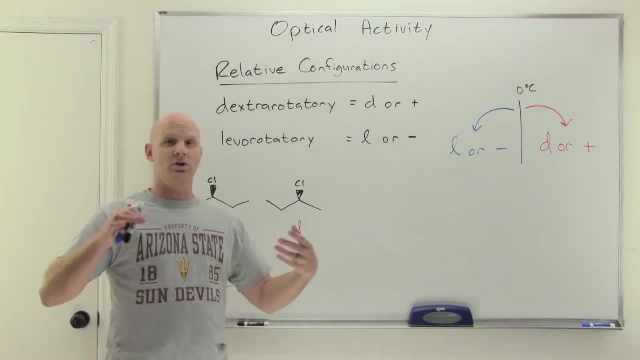 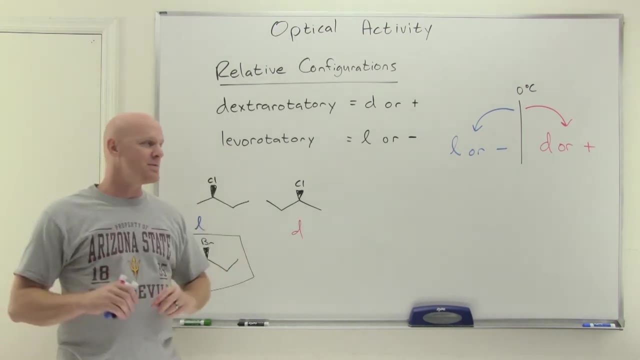 you know, a couple of guys got pretty crafty in what they did. But now that we've got NMR we can actually look and figure out which structure is which and which corresponds to which way the light is rotating and all that stuff. But up until you know, modern fairly. 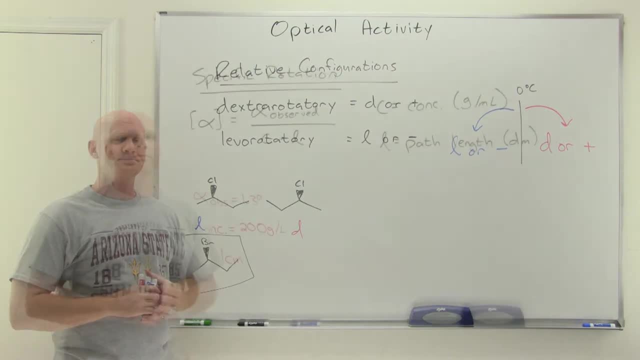 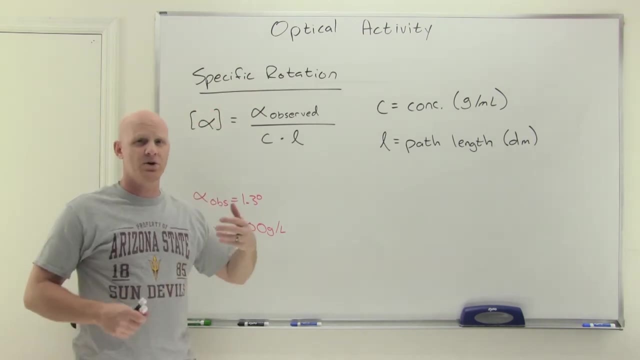 modern times. this was actually something that was rather challenging. All right, so now we want to talk about what's called the specific rotation, And it is something that is characteristic of a pair of enantiomers, And so that specific rotation will be one direction for one of the enantiomers. 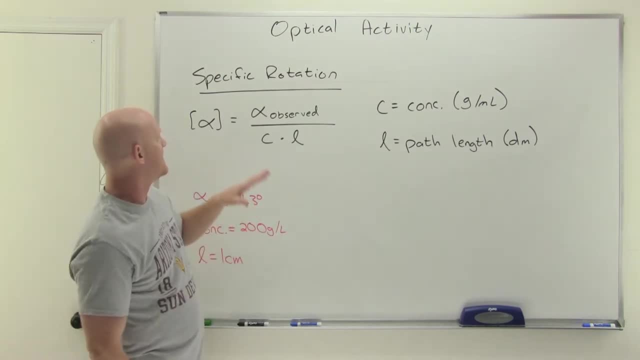 the opposite direction, by exactly the same angle though the other direction, And so that specific rotation is: just how far from the zero does this compound rotate for a given set of conditions? So it turns out, if you know you have a higher concentration of that compound, you get more. 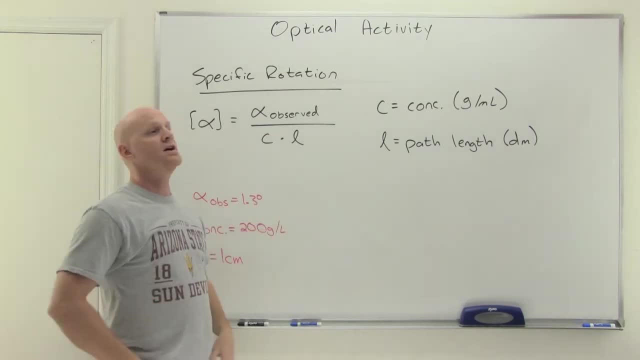 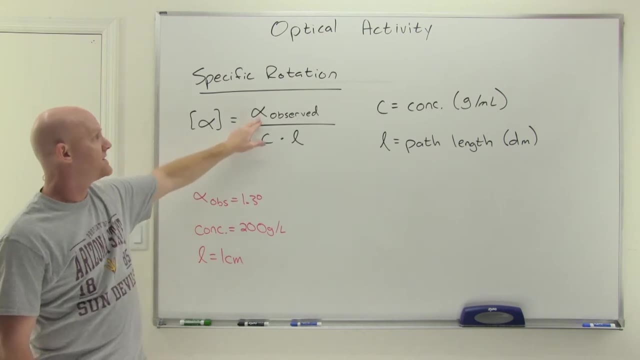 rotation. So if you have a longer path length which the light has to shine through, you're also going to get a longer rotation and stuff like this. And so what they do is they kind of scale it with this lovely calculation and they take the observed rotation for your specific solution and 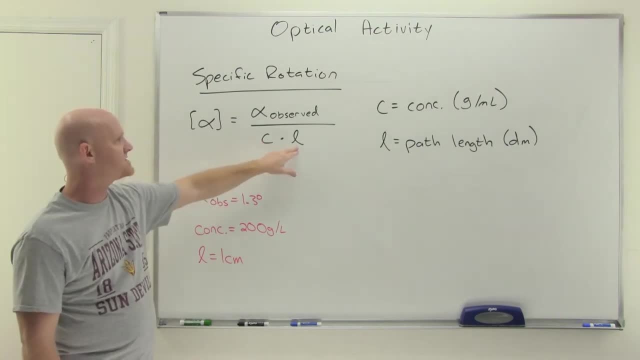 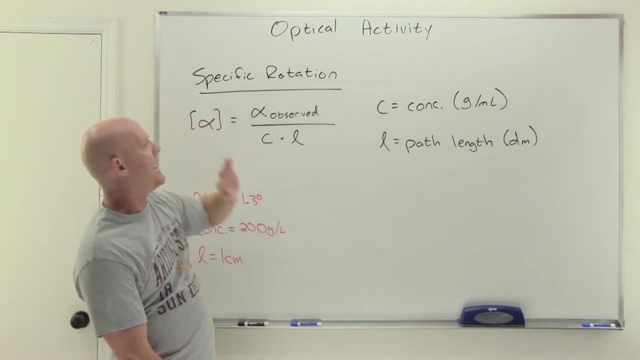 path length and stuff like that. But then they divide it To scale it by the concentration of path length. And here's where things get a little bit technical. That concentration, according to this formula, to get your specific rotation here, has to be in: 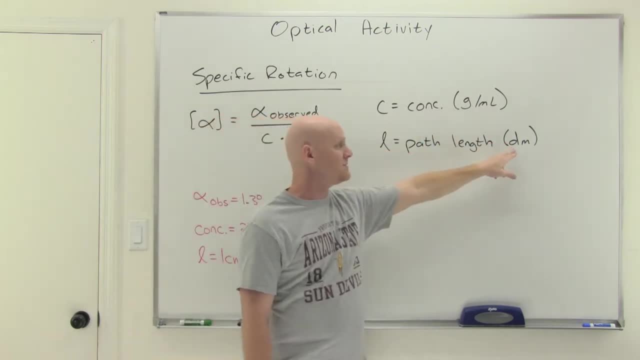 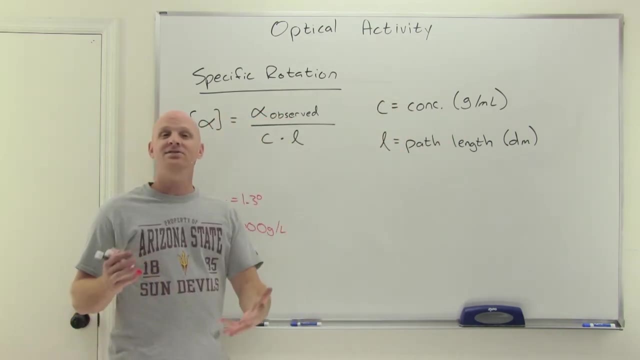 grams per milliliter And your path length- and this is horrible- has to be in decimeters, which we pretty much- I don't know of another place where we commonly use decimeters- So you should know that there are 10 centimeters in a decimeter, there are 10 decimeters in a meter, So that's where. 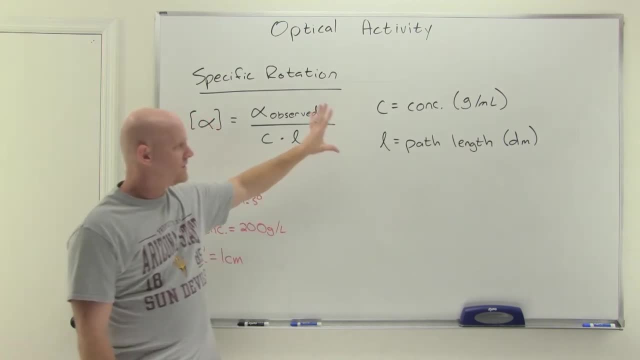 that decimeter falls right in between centimeters and meters- Cool, And so oftentimes this is one of the few places you're going to be able to do that. But if you're going to be able to do that, you're going to get a calculation here, And so we're going to do one ourself, And if you don't, 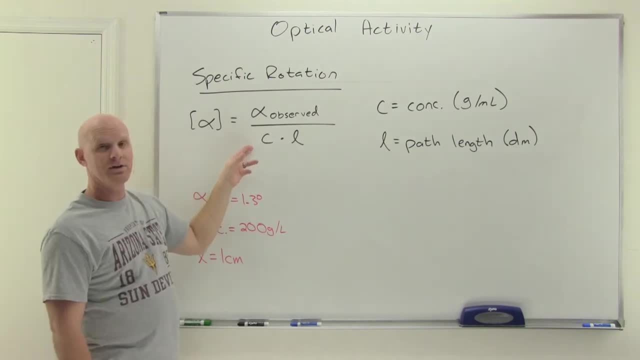 understand how these are defined and what units they are. you might not know how to plug them into a formula like this, And so in this case we want to calculate the specific rotation. when the observed rotation is 1.3 degrees, And notice that's positive 1.3 degrees, which means to the right. 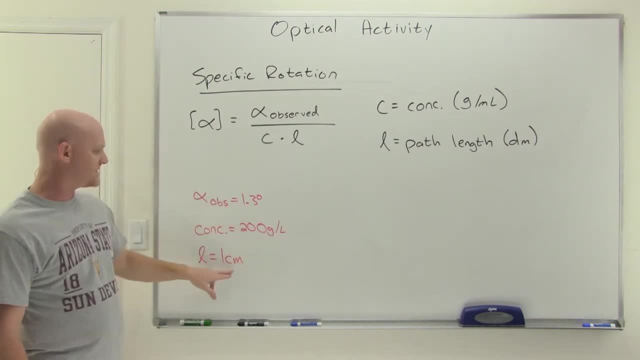 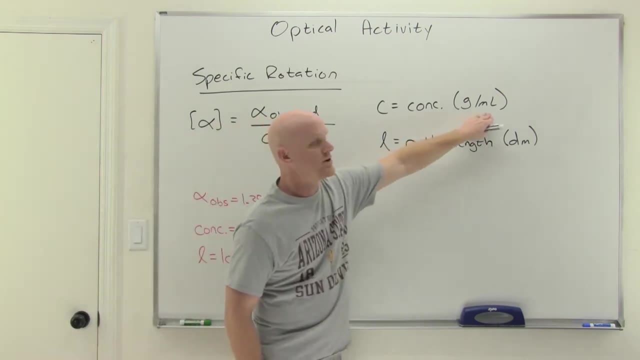 So concentration is 200 grams per liter and the path length is one centimeter. And one thing: you should realize that neither one of these units is correct. So 200 grams per liter. Well, if there's two of them, you're going to get a calculation here, And so we're going to do one. 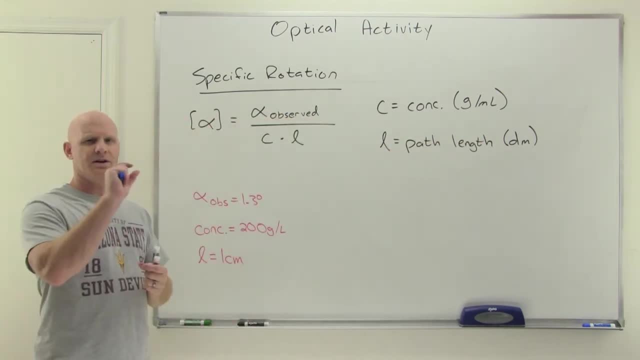 centimeter. Well, if there's 200 grams in a whole liter, well then, how much is in a little milliliter? Well, a milliliter is only one one thousandth of a liter. So if there's 200 grams, 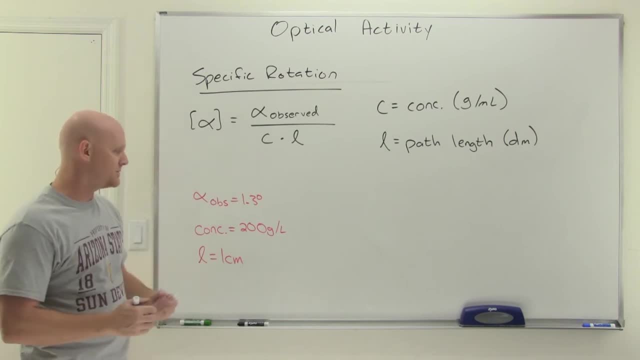 in that big old liter. there's going to be a thousand times less in that little milliliter, And obviously you could do some dimensional analysis and do the calculation here. But I'm going to reason that out, And so in this case this corresponds to 0.2 grams per milliliter. 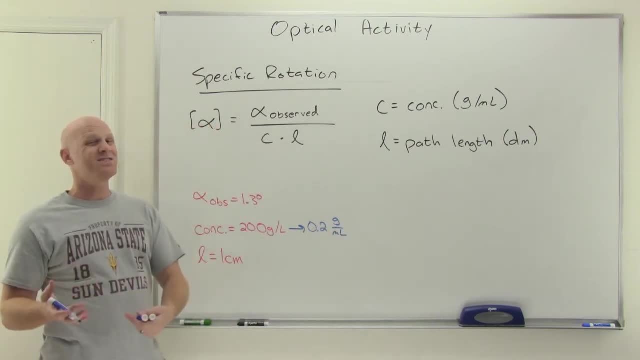 That's what will actually go in the formula here, And then one centimeter again. there's 10 centimeters in a decimeter, So this would correspond to one tenth of a decimeter, And that's what, once again, will get plugged into our calculation. 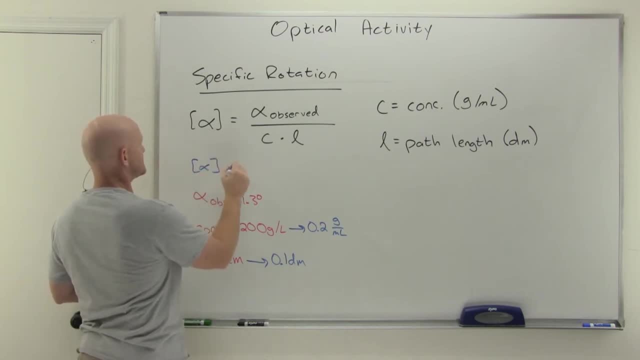 So, and here we'll go. So our specific rotation would equal 1.3 degrees all over, a concentration now of 0.2 grams per milliliter and 0.1 path length, 0.1 decimeters. Cool, And because these 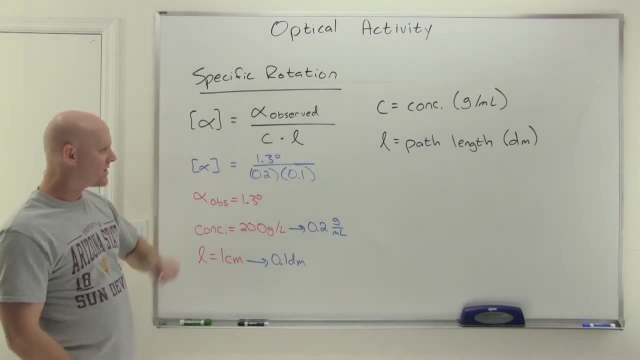 are the right units. I'm just going to leave this off, And we look at this as kind of being a unitless term here Just has or shouldn't say unitless, but just degrees, All right. But again, these do have to be plugged into the correct units And from here I'm going to use my handy. 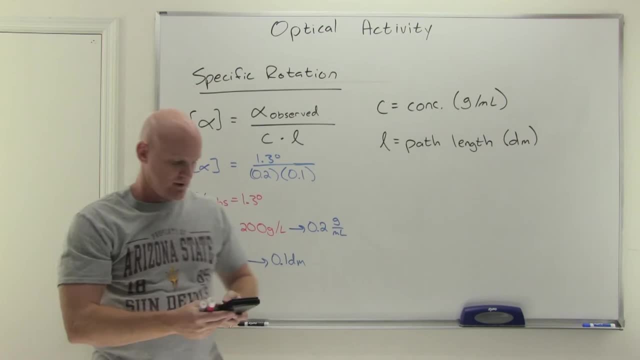 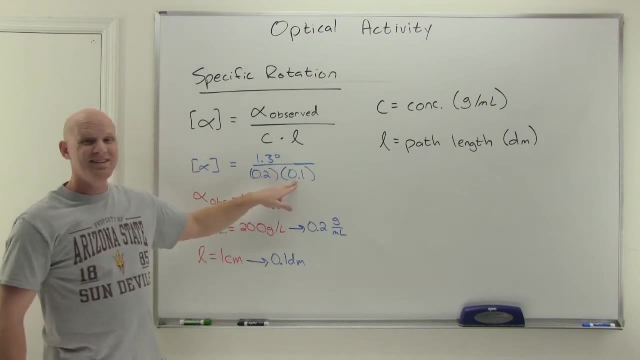 dandy calculator. So I definitely don't feel like doing this in my head, but we could right. So, if you notice, actually we'll just do this in our head, Why not? So dividing by 0.1 is the same. 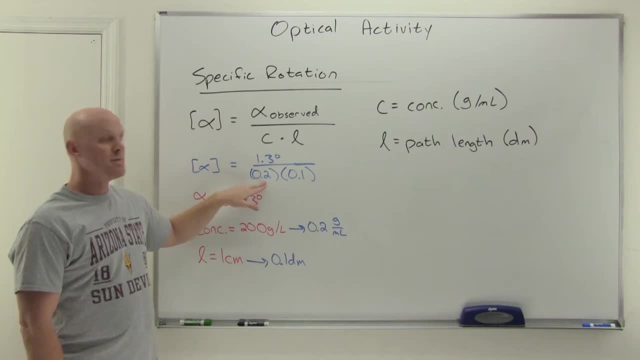 thing as multiplying by 10.. That's going to take this up to 13.. Dividing by 0.2, which is one fifth, is the same thing as multiplying by five, And so really, we're just going to end with five times. 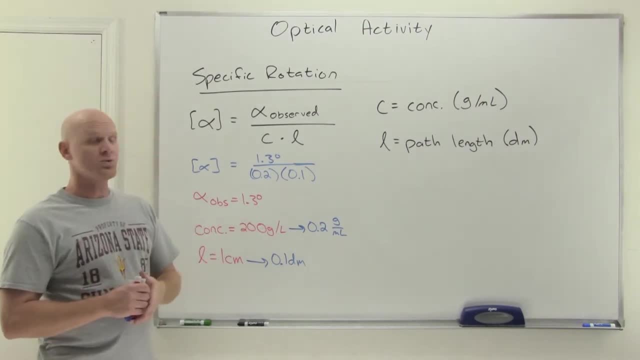 13.. Five times 10 is 50, and five times three is 15.. So we're going to get 65.5.. Degrees here, Cool, One of the few places in all of organic chemistry where you might see a calculation. And again, I gave you the numbers. They're not too terrible. Obviously, we did this. 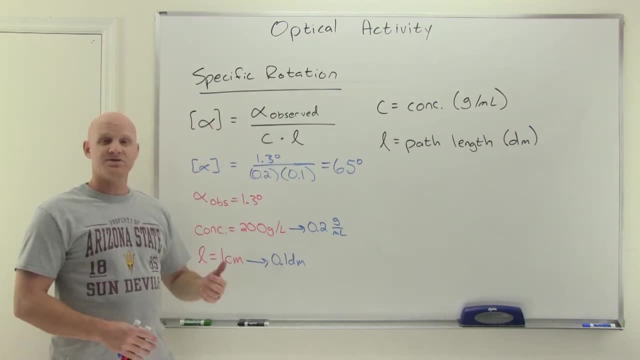 in our head. But obviously your professor's either got to have you come prepared with a calculator or sometimes they'll just say: you know what, Just set up the calculation Don't actually solve, Because most of the time we're not going to have you guys bring a calculator to. 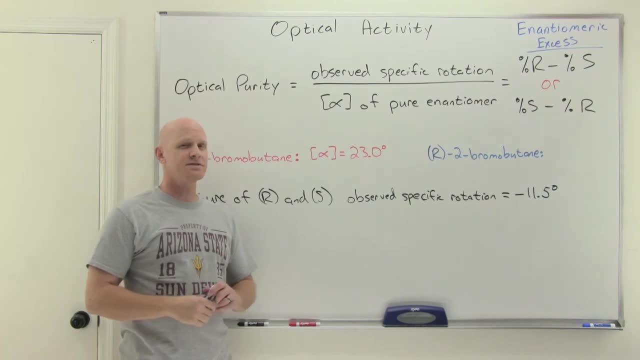 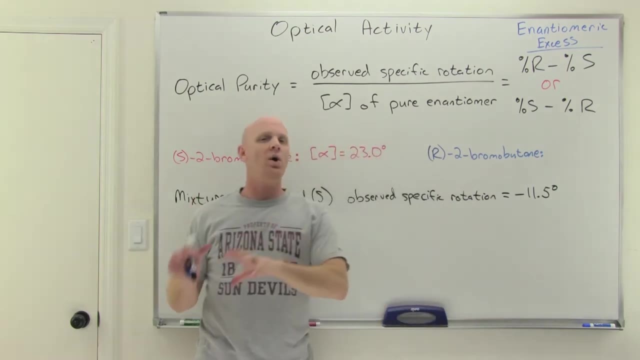 an O-Chem test, All right. So last little section in this lesson. we're talking about optical purity and enantiomeric excess. So this is when you've got both R and S enantiomers, a pair of enantiomers. 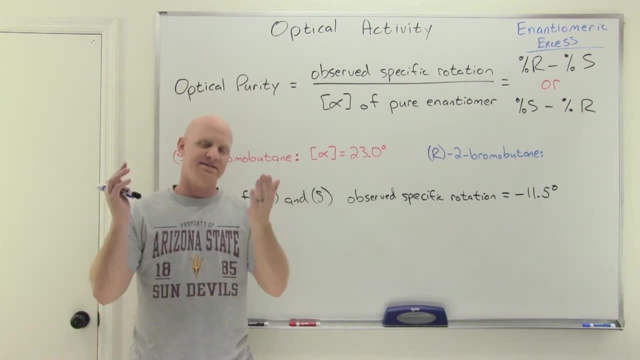 mixed together. Now, if they're mixed together exactly 50-50, that's a racemic mixture and it's going to be optically inactive. But now we're going to treat with. what do you do if it's not exactly 50-50?? What if it's 51-49?? What if it's 75-25?? Something like this Then: 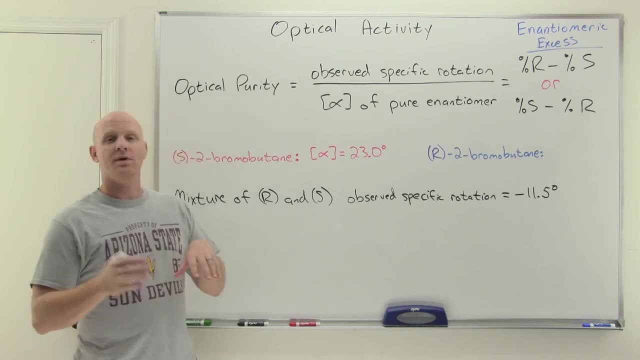 that solution will be optically active And so we can figure out what that rotation might be, or figure out, based on the rotation, what the purity is and things of this sort. We're going to take a look specifically at an example of S2-bromobutane And for pure S2-bromobutane. 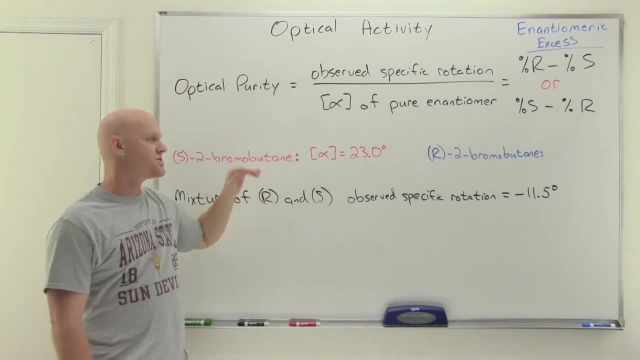 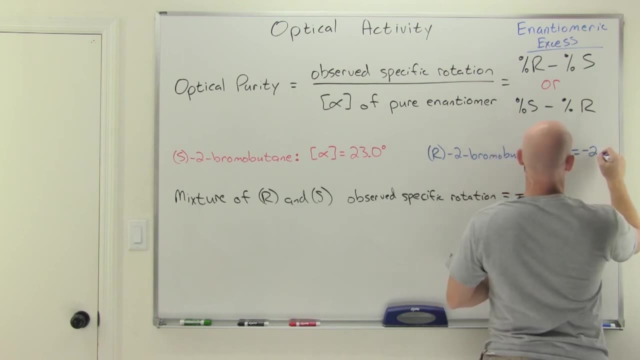 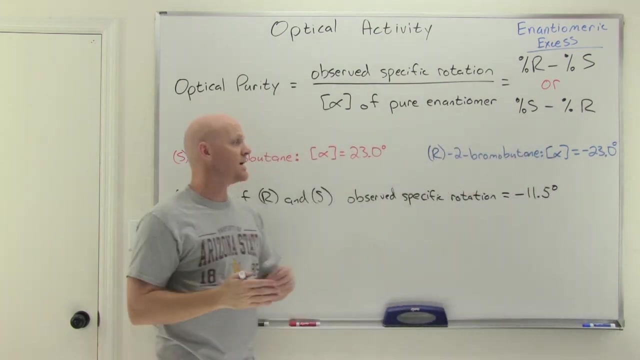 its specific rotation is 23 degrees. What you should know, then, is that if I've got R2-bromobutane, its specific rotation would be negative 23 degrees. Let's get a decimal place in there as well. So negative 23 degrees, Okay, great. So this one's given, this one's just inferred. 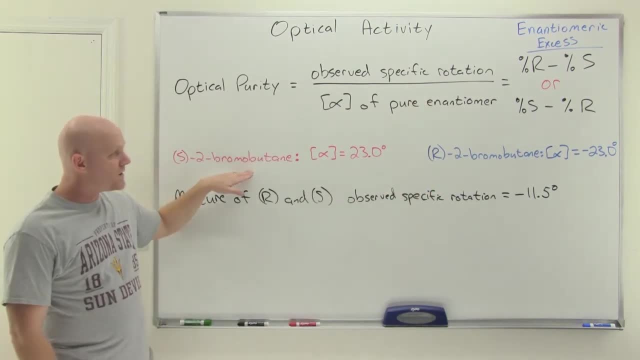 It's the exact opposite direction for the enantiomer. So once you're given one, you know the other is the exact opposite. Cool. Well, we're going to have a mixture of both R and S2-bromobutane mixed together, So in that mixture we get an observed specific rotation of negative. 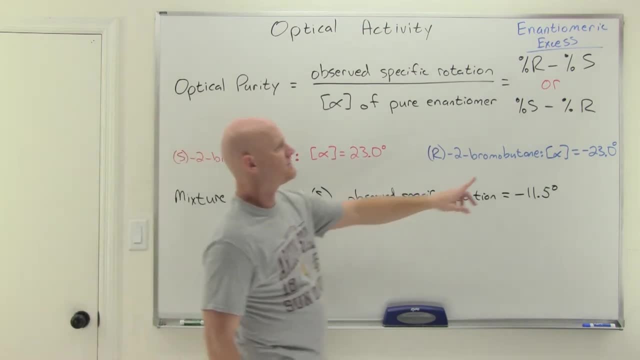 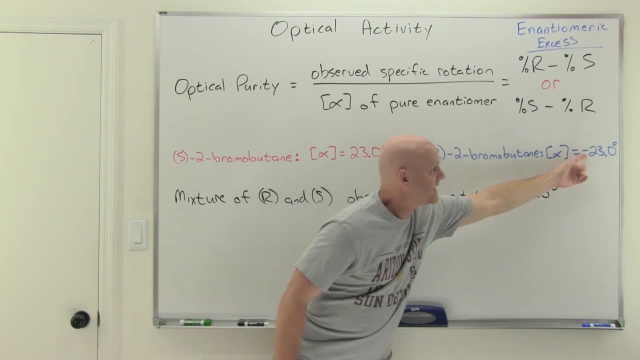 11.5 degrees. Now because it's negative. we can infer that in this example there's more R2-bromobutane than there is S2-bromobutane. So because it's got a negative observed specific rotation The. 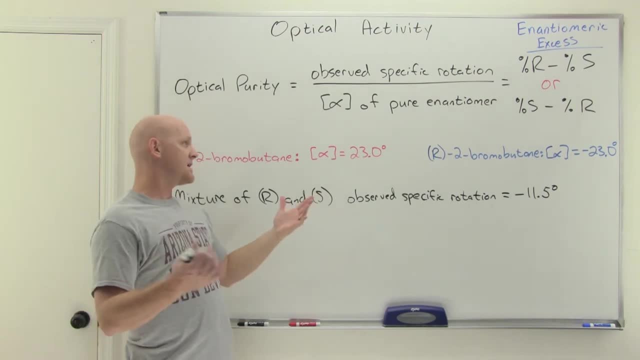 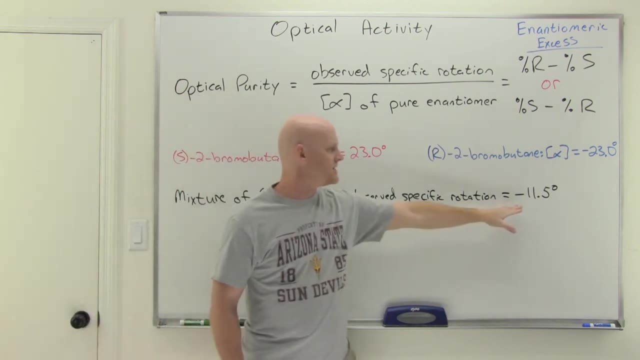 question, though, is that: what is the composition of that mixture? Okay, Well, once again. so we're going to take a look at this optical idea of optical purity, and we can figure out what that is based on the observed specific rotation of the mixture, and what the specific rotation is for. 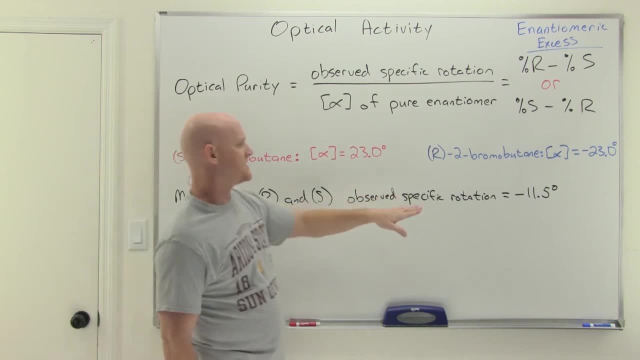 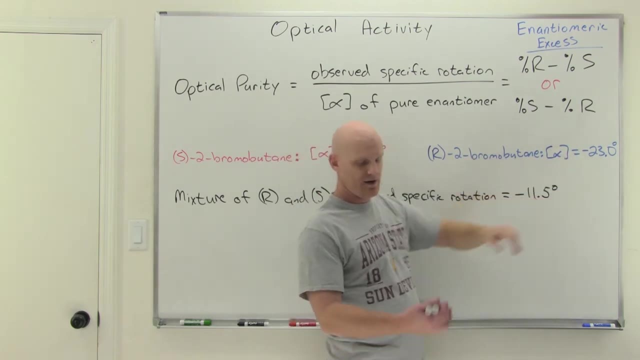 either pure enantiomer. So in this case I can see the observed specific rotation is negative 11.5.. I'm going to choose to compare that to the pure R2-bromobutane because it's also negative, And so in this case our optical purity, which I'll just call OP, equals negative 11.5 degrees. 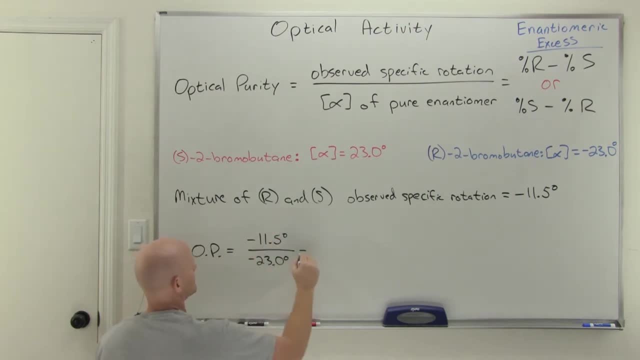 all over negative 23.0 degrees, And we'll see that this is going to exactly equal 0.5.. Okay, So that's our optical purity. Well, it turns out your optical purity equals your enantiomeric excess as well, And so your enantiomeric excess here. so it's just how much more of one enantiomer? 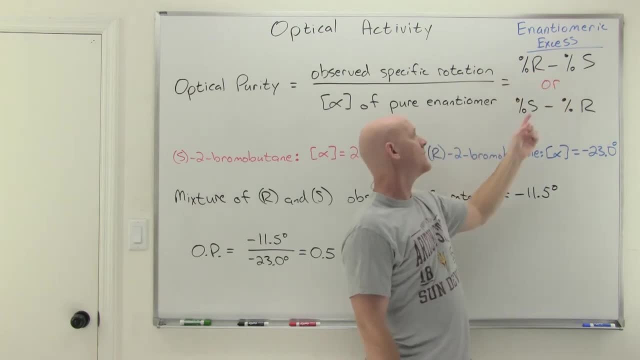 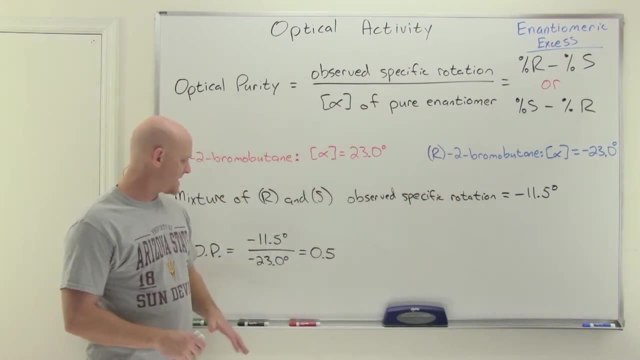 you have than the other. So it's either percent R minus percent S if you have more percent R, or it's percent S minus percent R if you have more percent S. Well, in our case, we definitely know we had greater percent R, All right, So in this example, 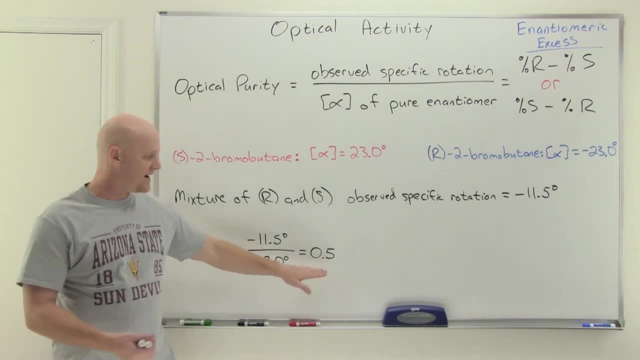 with an optical purity of 0.5, what this tells us as a percentage, this corresponds to 50%, So keep that in mind. So in this case, our optical purity means that our enantiomeric excess is also 50%. 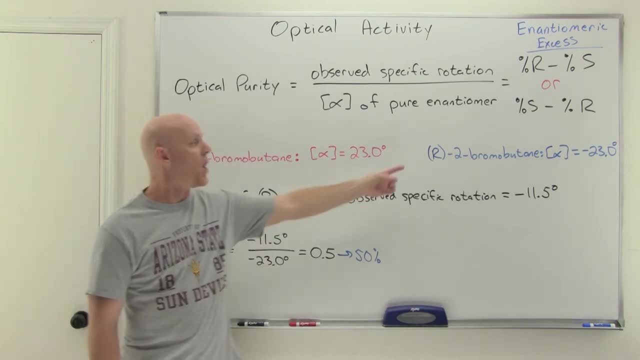 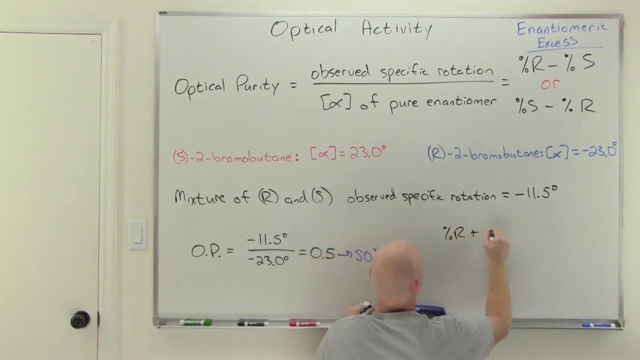 There's 50% more in this case R than S, And so we can figure this out then, because we know that the percent R plus the percent S has to add up to 100%, So they got a total up to all of it, But now we know that. 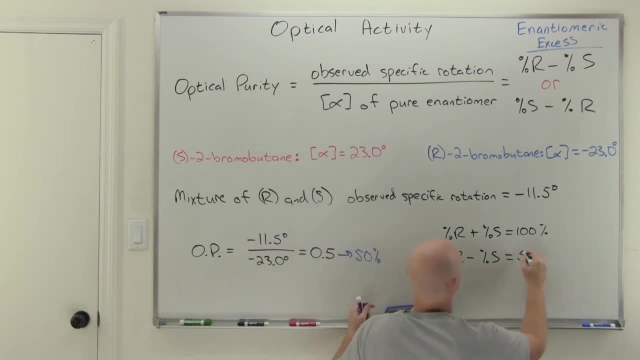 the percent R minus the percent S equals 50%, And now we have two equations with two unknowns and we're going to have to solve. So take a look here. There's a couple different ways you can approach this. I personally just like doing linear combinations, sometimes called elimination. 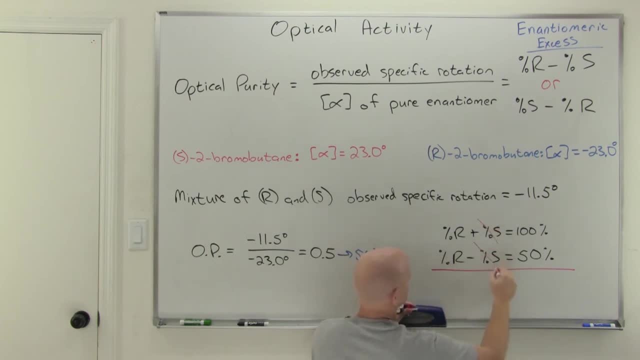 because if you just add these together, notice the percent S are going to cancel, Plus percent S, minus percent S. add it together, they're gone, And so you end up with two times the percent R is going to add up to 150% And we find out that our percent R when we solve. 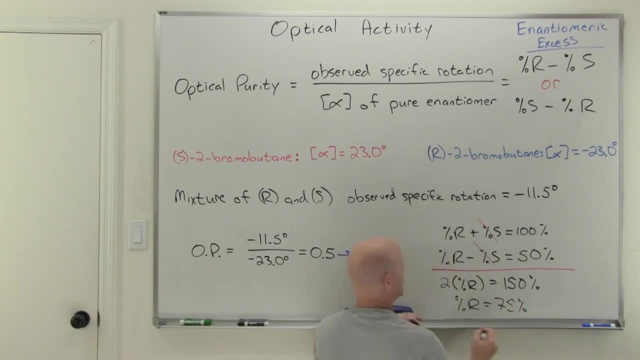 for it. divide by two equals 75%, And if the percent R is 75%, the percent S must have been the rest, So 25%. And so we can see: yep, they both add up to 100% And there's 50% more R than. 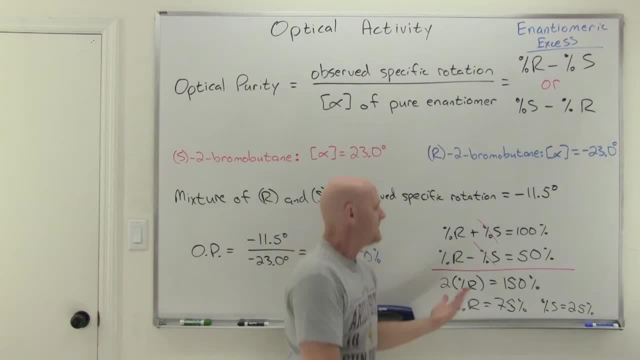 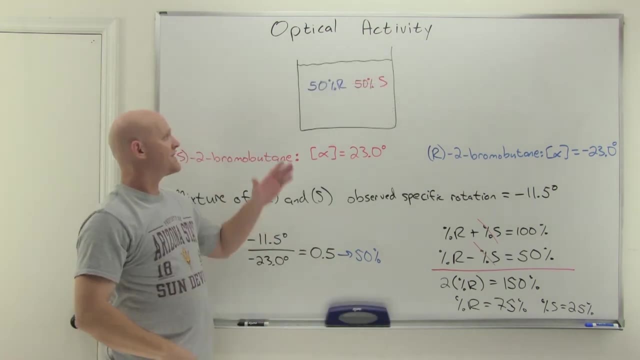 they total 75% minus 25% is 50%, And so this matches all the numbers. Now let's take a little closer look at what's really going on in this solution. All right, so let's go back to that racemic mixture. If we had 50% R and 50% S, then, as a result, their specific optical activity would 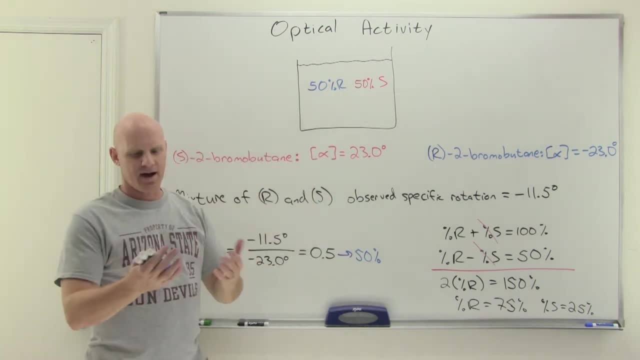 cancel each other out and that racemic mixture would be optically inactive. Well, that's not the case that we had in this example. We instead had 75% R and 25% S. So let me lower that percent S. 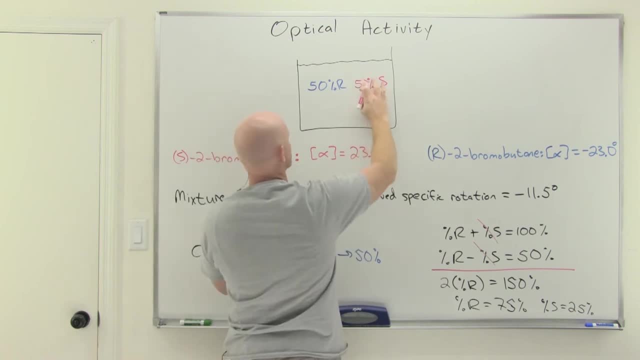 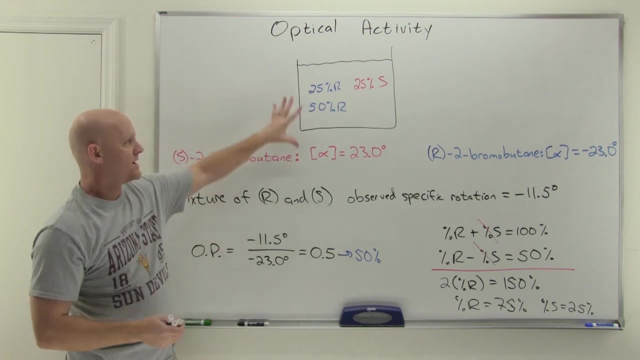 percent r and 25 percent s. so let me lower that percent s down. we're gonna lower that down to 25, so, and the percent r goes up to 75, except i'm gonna leave that looking like this. i'm gonna put break it up: 25 r plus another 50 r adds up to a total of 75 r. and the reason i did this is because 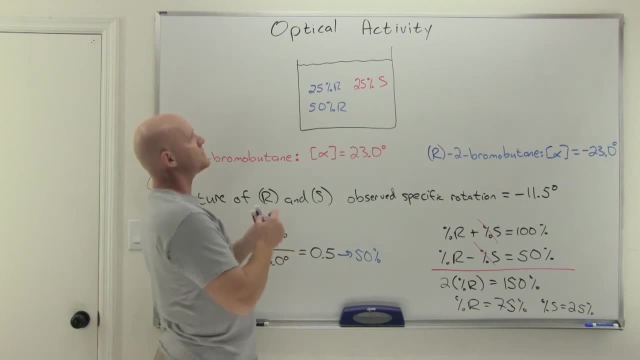 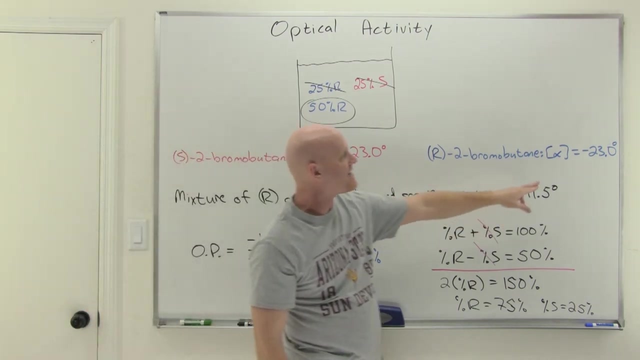 the 25 percent s effectively is canceling out the rotation caused by the 25 percent r. they cancel each other out, and so what you're left with is that 50 percent uh of the solution that's left over that's not cancelled out is still r, which is why it gives half the rotation of what pure r is. 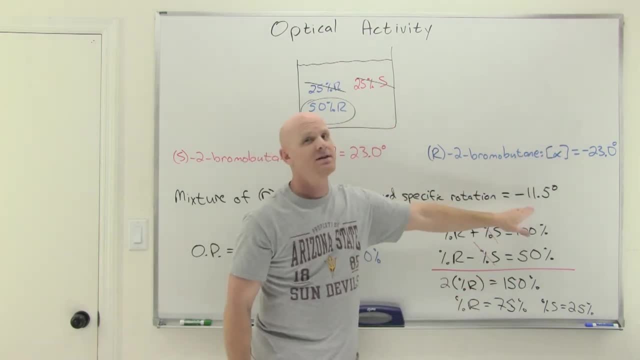 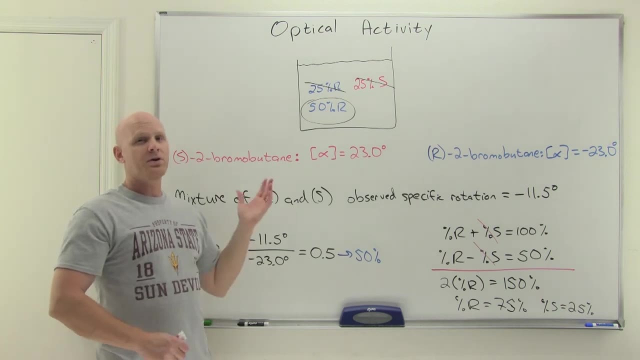 going to do, which is where that negative 11.5 degrees came into play. so that's really what's going on. just wanted to see it from this perspective. so sometimes we'll give you the uh optical purity and have you figure out what the rotation is going to be. sometimes we'll give you 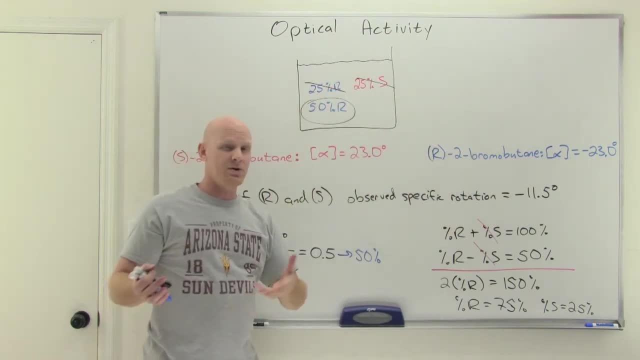 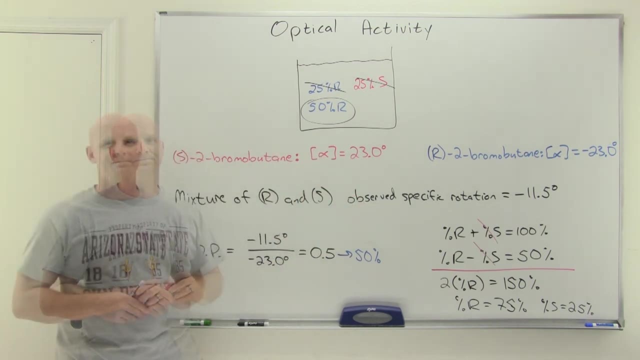 that observed split rotation and have you go back and figure out what the optical purity and an antimeric excess would be instead, but once again, that optical purity and antimeric excess are always equal to each other. now, if you benefited from this lesson, consider giving me a like and 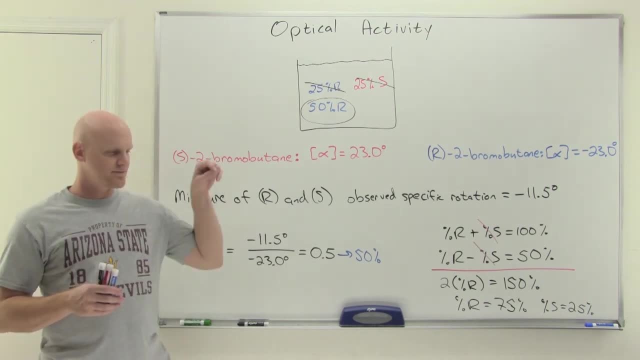 a share- one of the best things you can do to support the channel- and if you've got questions, feel free to leave them in the comment section below. if you're looking for the study guides that go with this lesson, or if you're looking for practice problems, check out my premium course. on chad's prepcom you.